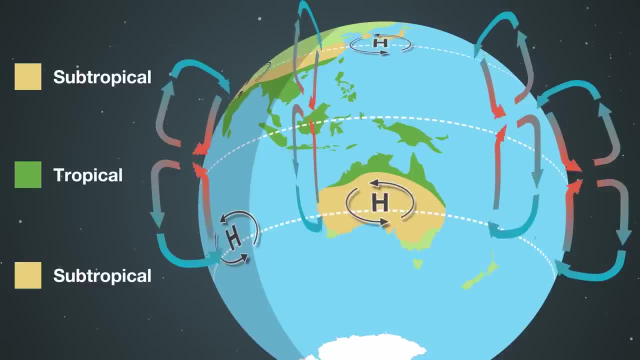 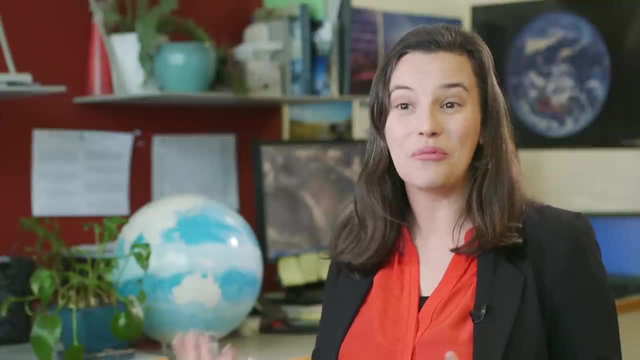 the air from the tropics falls as dry air. The sinking air makes for high pressure systems and clear skies at the earth's surface, so the subtropical zone is fairly dry. Places like Longreach and Brisbane are considered subtropical. The summers are hot, the winters 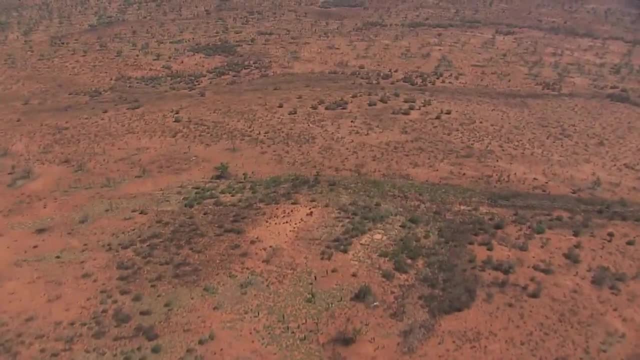 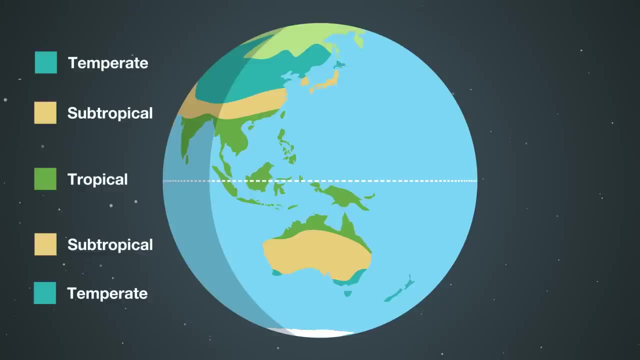 are mild, And the subtropics is where we currently have most of the world's deserts. The next climate zone is the temperate zone. Because the earth is round, sunlight hits these areas on more of an angle than at the equator. The same amount of energy then has. 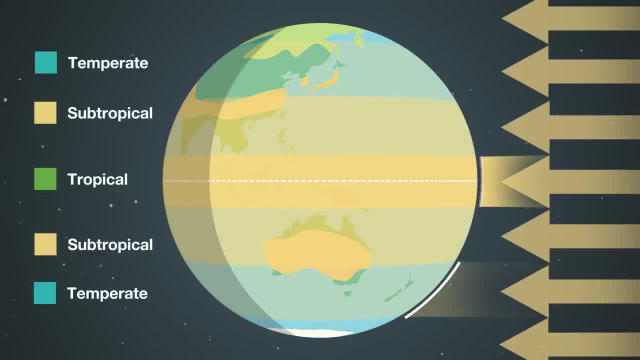 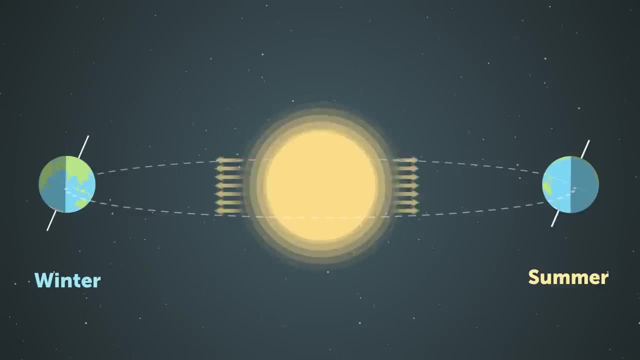 to cover a larger area, which means it's cooler here than at the tropics, And because the earth is tilted as well as we move around the sun during the year, the temperate zones receive less direct sunlight in winter and more in summer. 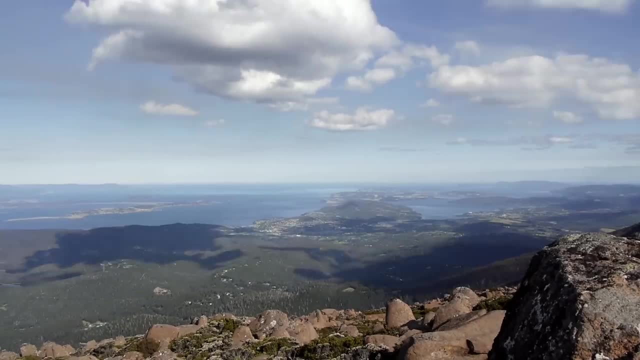 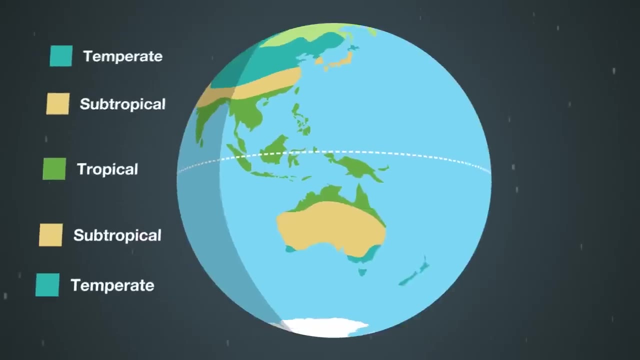 Regions in the temperate zone, like Hobart and Melbourne, therefore have distinct seasons – with cold short days in winter and warm long days in summer. The coldest climate zone is the polar zone. Here the sun is lowest in the sky and its 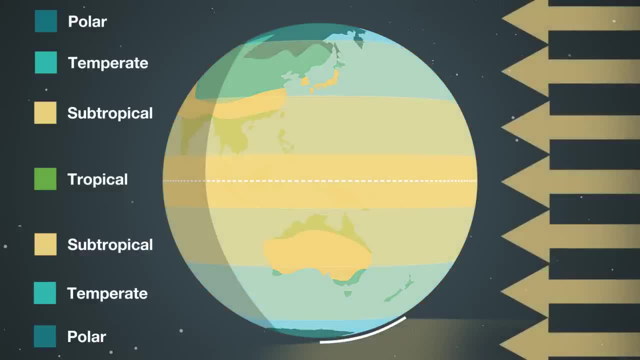 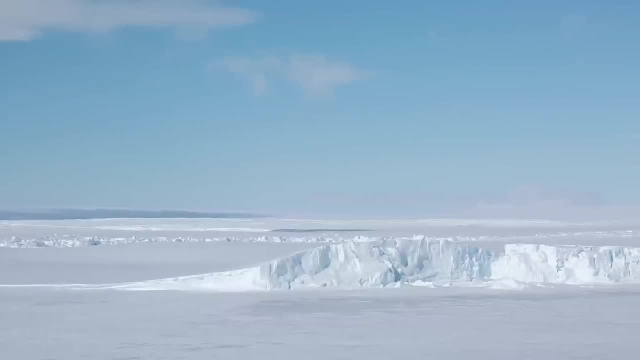 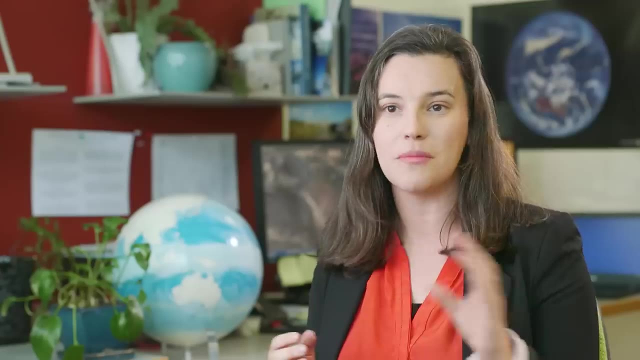 rays and energy reach the earth at an even larger angle. The polar zone is very cold and cold air can't hold a lot of moisture. Some areas in the Arctic and Antarctic are as dry as our subtropical deserts- enough to experience the tropical zone in the north, the subtropical zone across. 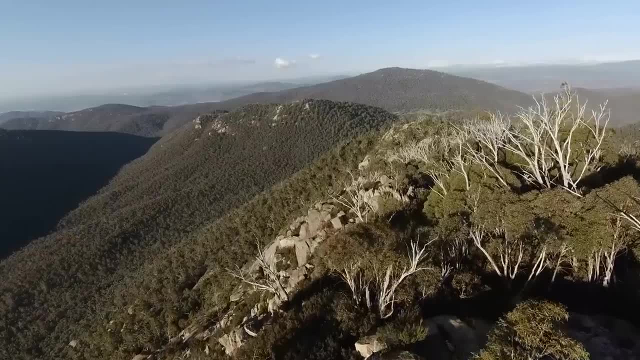 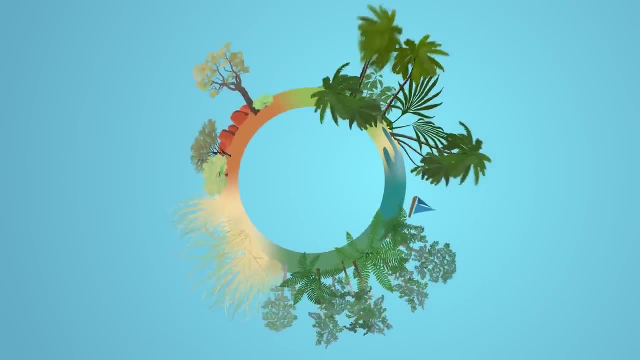 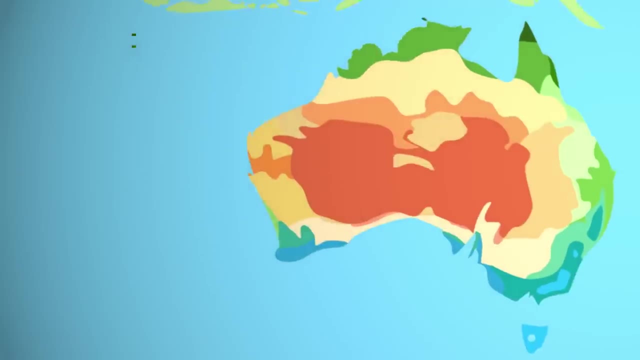 much of the centre and the temperate zone in our south. Other features, such as our mountain ranges or how far places are away from the sea, can make things a bit more complicated, and you can break these zones up into sort of sub zones based on temperature, rainfall and vegetation that grows. The Great Dividing. 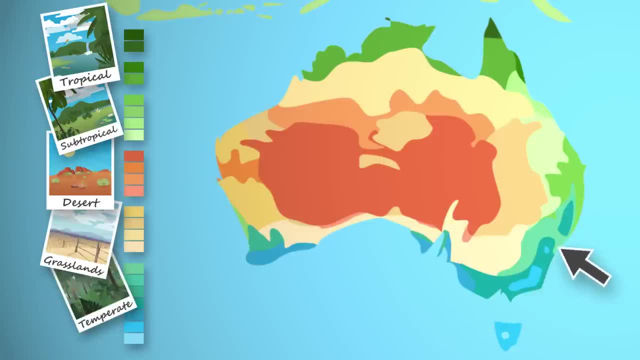 Range, for example, helps the temperate zone reach up along the east coast of New South Wales. Our red centre is mainly classified as desert, while coastal regions at a similar latitude are considered subtropical or grassland. Australia is one of only a few countries that spans multiple climate zones, so be sure to make the most of it.